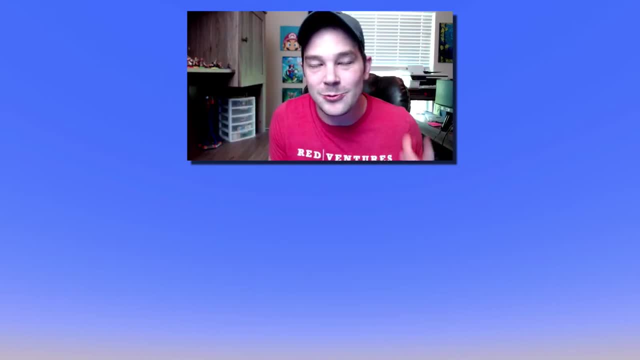 things with the GPU that are outside of the box of graphics. You don't need to do graphics, and that's what I'm trying to get across to you during this episode. So let's go about using metal or the GPU to execute our functions, as opposed to the CPU. This is going to be great. I hope you guys really. 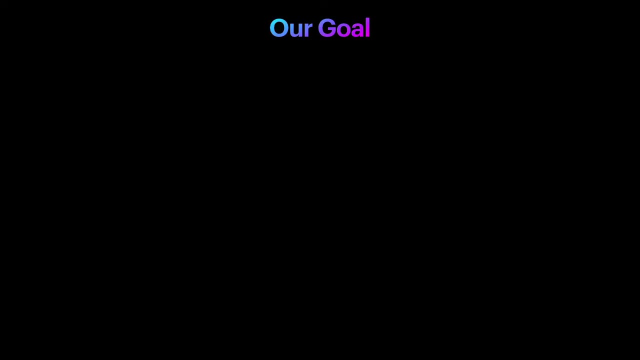 enjoy this episode. Let's go So in order to explain to you exactly how to use compute functions. what we're going to do is we're going to use a very simple example, which is just taking two different arrays. In this case, it's just seven different data points, adding them together and 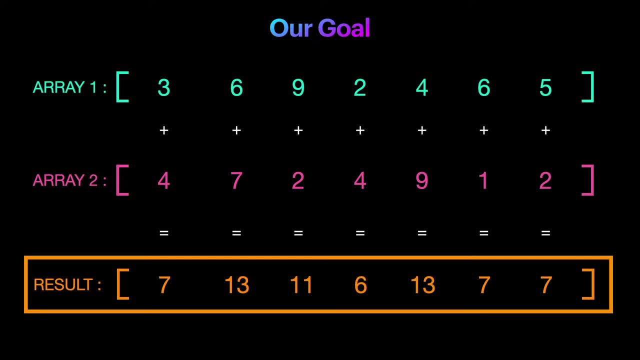 getting a final resulting array with all of those indices kind of added up together individually. Now I know this may sound a little bit boring, but I promise you the result is going to be awesome. You're going to see a really huge optimization happening with our applications. 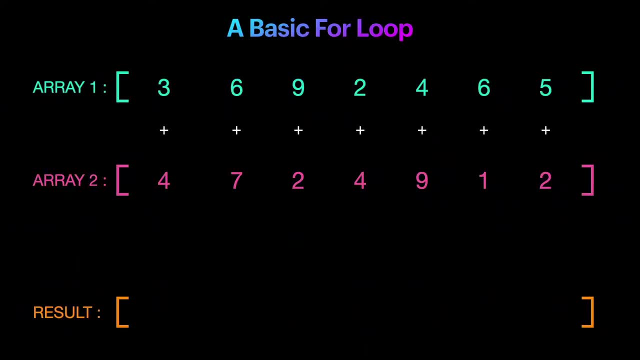 So let's talk about our basic for loop, Like how I would solve this If I was just using a CPU single encoded operation. I would just use a for loop, So I would go into C by end to C. I'd say this index. 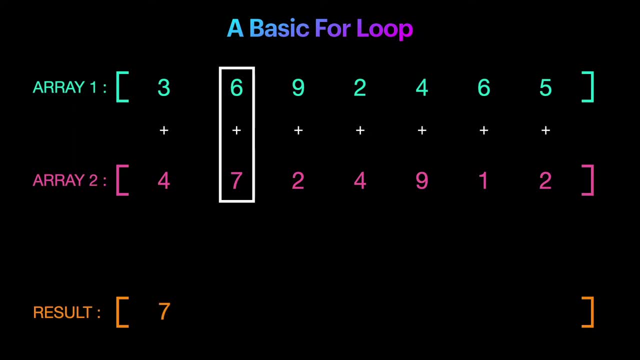 add them together, get a value store that as a result, I'd add this next value together, These two seven plus six, get a result store that in the result array. And then I would continually do this all the way down the line, one after the other, until I finally have a result array Now. 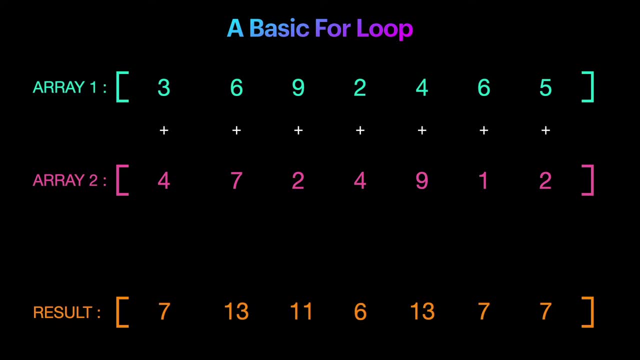 I'm working with seven different points here, So it's very small. but say we're working with these- array one and array two being like I don't know a million data points. That's where this is going to slow down And that's where you can get into like the big O. 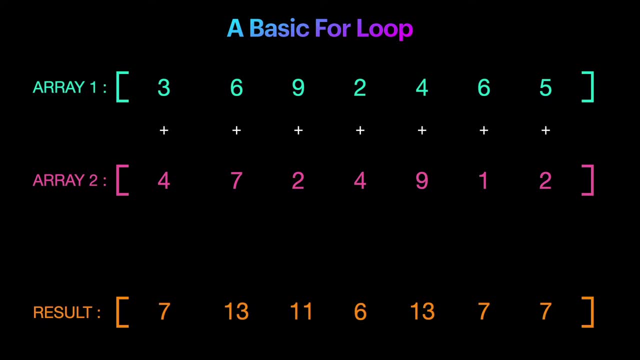 factor. We're not going to do that in this episode. Basically, this is good for small data sets, but if we are growing into millions of data sets, that's when we want to do: use a better approach, And this better approach is instead of processing one at a time, like three plus four, six plus seven. 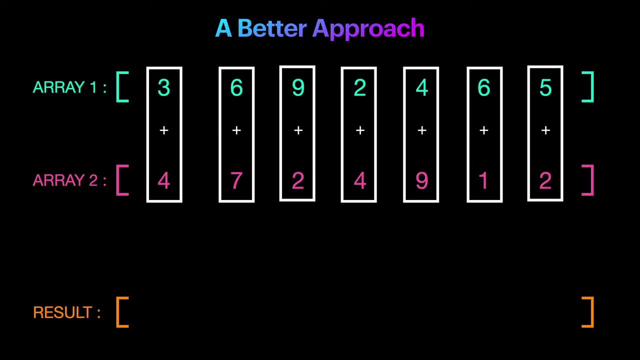 we are going to be doing every single one of them at the exact same time, using one thread, So every single one of these operations is going to have its own individual thread, And then what we're going to do is we're going to bring it all together at exactly the same time and create this. 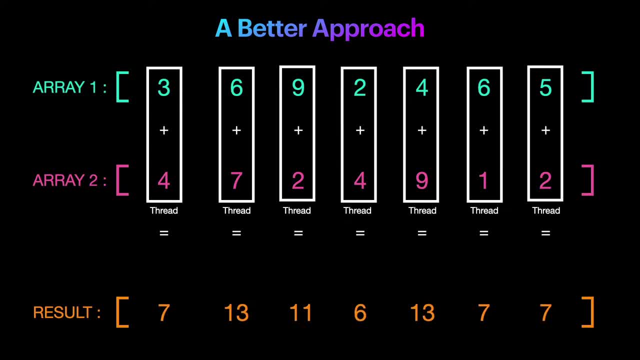 resulting array. So, as you can see, this goes a lot faster than just adding each individual index at. you know, one after the other, it's, it's. this is going to be way faster, So let's show you how to use the GPU. All right, So I'll be working with a brand new application. I'm going to create a. 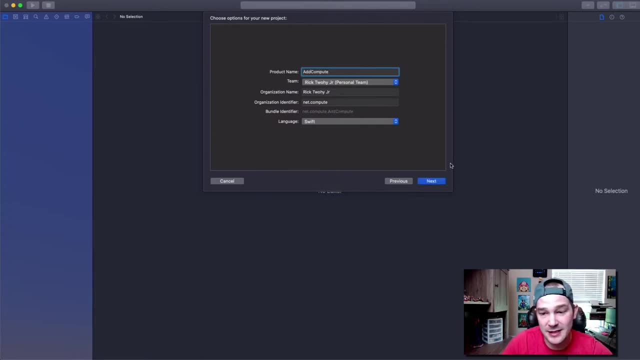 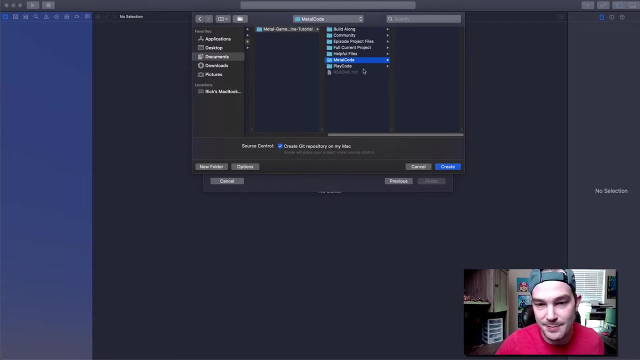 command line tool. I'm going to call it add compute, and then I'm going to save it. Now, where I'm going to save it is I'm going to save it To my GitHub, So you can go and get this if you want. Um, I'm going to put it inside this metal. 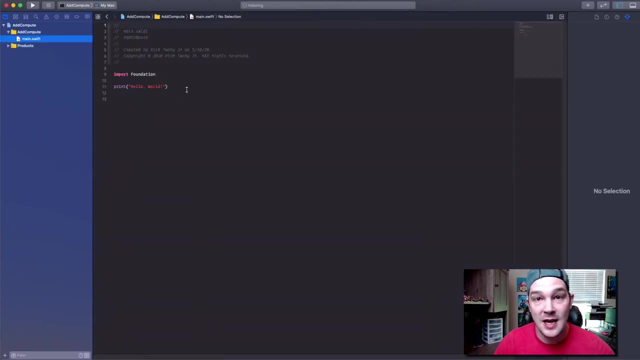 code folder and I'm going to create it. And now we have our new project. If we go into this main dot Swift file, you'll see we have all of this stuff. That's kind of auto-generated. I don't need that. All I need to really do is import my metal kit, Cause that's what we need to work with. 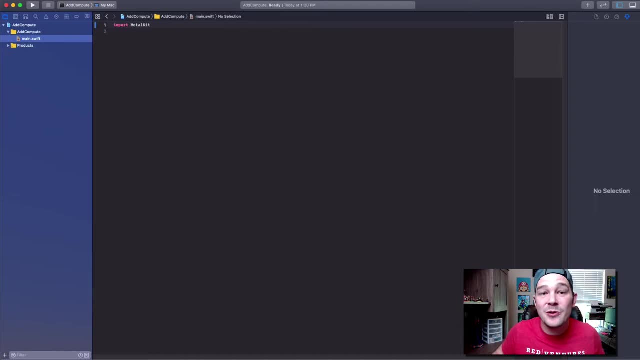 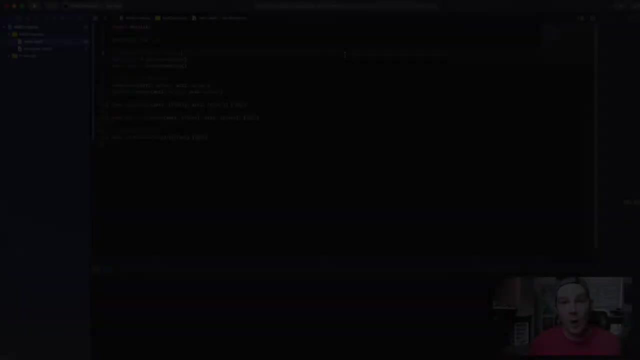 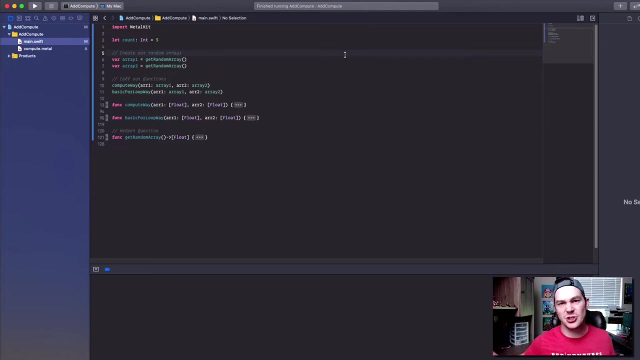 need to fire up a cocoa application. I can do this simply with the command line tool. Okay, So fast forwarding into the future. I've already recorded everything and then I edited it. That's way too long, So what I'm going to do is I'm just going to shorten this down, If you want me to post. 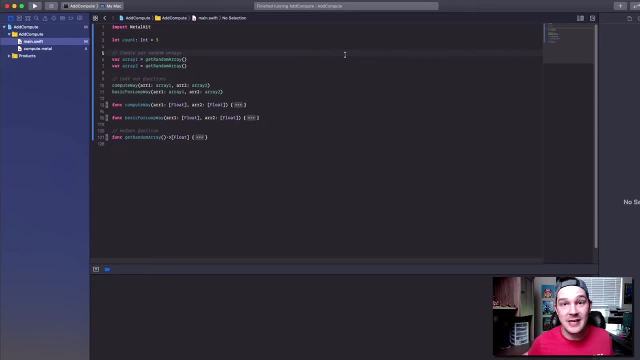 all of the line by line descriptions. you let me know I will post that video as well, but for now let's just talk about the code. I did because this should be way faster and this might give you a little bit more value. So let's dive into it, Starting at line three. we have a count Now. 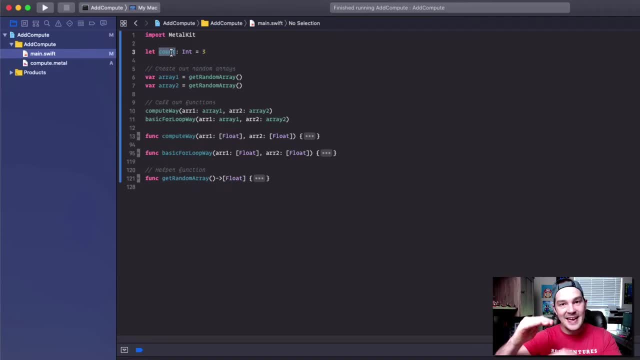 this count represents how many items that we're going to be putting in the array. Okay, Then we're creating two different arrays to add together based on this function get random array. This get random array basically creates this empty result array based on that count. 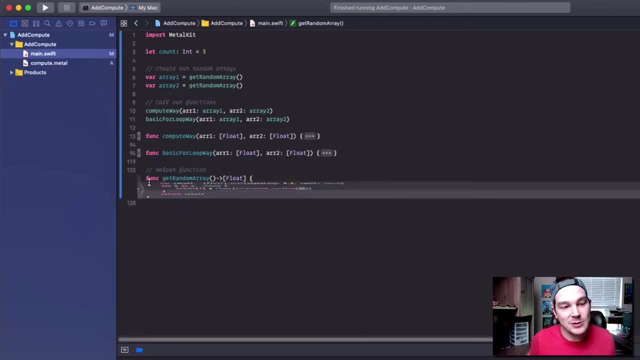 and then fills it up with random numbers and then it returns that value. But that's what the get random array does. So we're generating two different arrays based on this count. The next thing we're going to do is we're going to call compute way. So this is going to be. 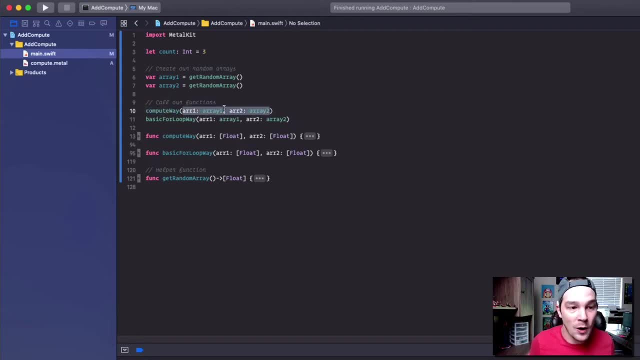 like our compute GPU way and we're passing in array one and array two And then this is going to be the basic for loop way. So this will take in also array one and array two. So this is going to be GPU, this is going to be more CPU processing And, as you can see, 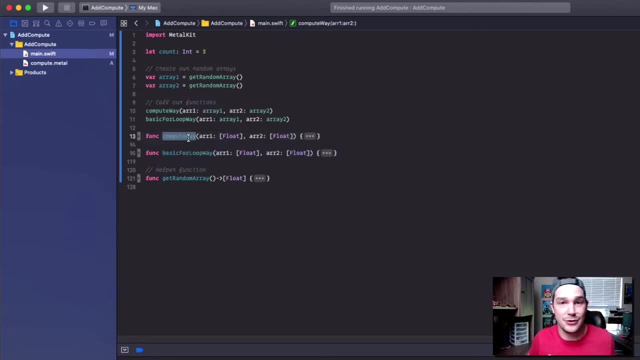 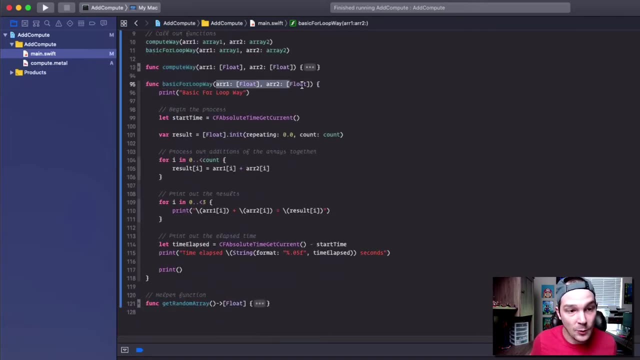 I've defined both of those functions right here Now. I'm not going to talk about the compute way function yet. We'll get into that in just a little bit. What I do want to talk about is this basic for loop way that takes in array one and array two. Now, inside of here, 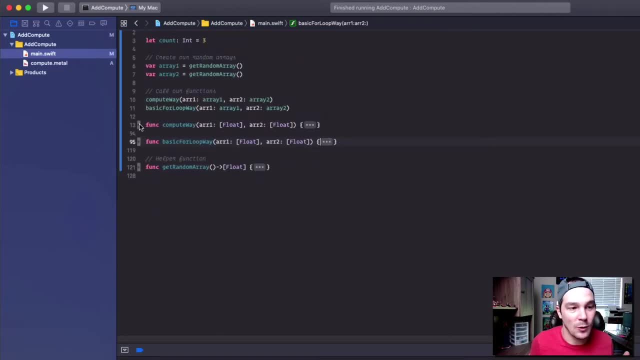 And I do basically the same thing in the compute way, except the compute way is a little bit more complicated, And we'll get into that in just a second, But for now let's actually run this and see what kind of results we get. So if I were to bring this up, 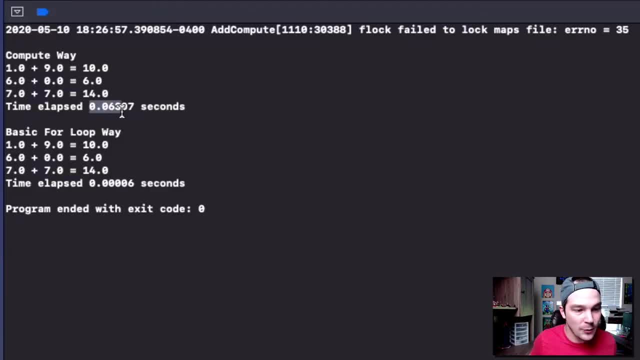 as you can see, when we run the compute way, we get 0.063 seconds. And then, right here for the basic for loop way, we get 0.0006 seconds. Now you're probably thinking yourself: okay, well, the for loop way was way faster, holy hell, was that faster? But just know. 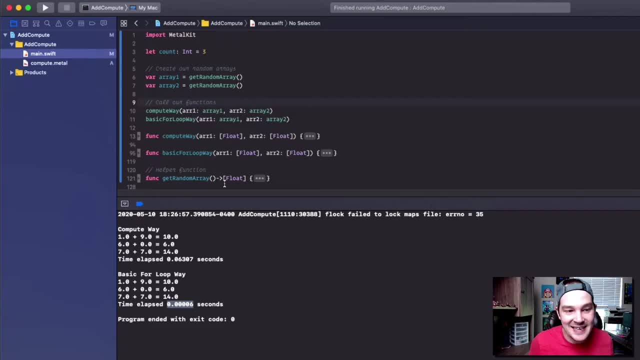 this is actually really important to know. we might not actually need to use the GPU for every single thing. If we're using a for loop that has three values in it, don't use the GPU. that's wasteful. You don't need to because obviously it's way faster just to use a basic. 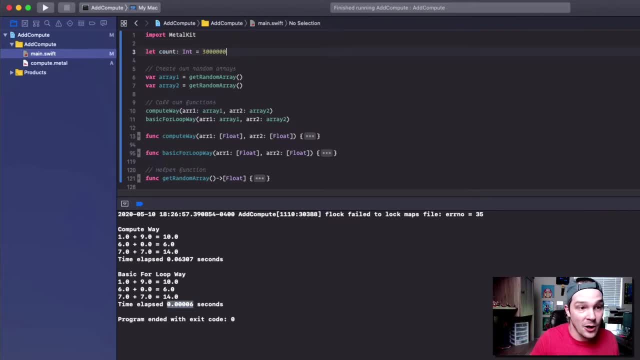 for loop. Now, if we were to increase this number to something like I don't know 3 million and then run it, let's see what the result of that would be, And, as you can see, we have a big difference. 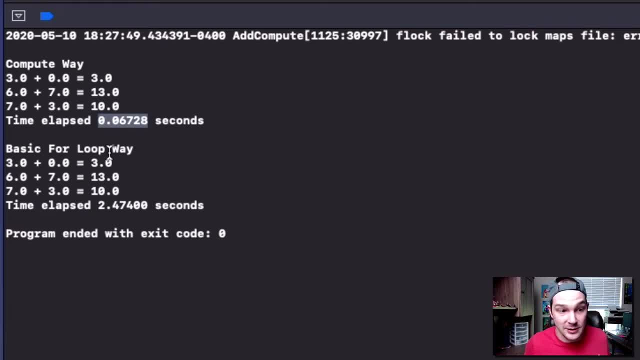 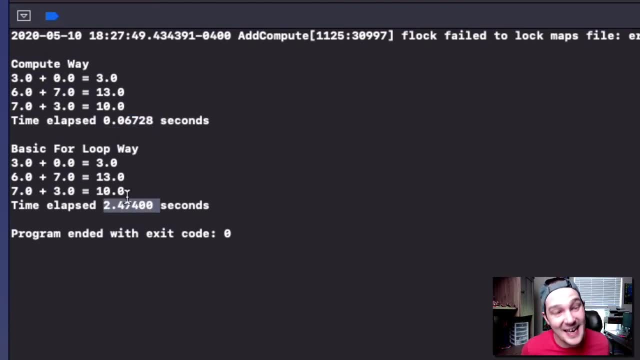 Now the compute way has basically stayed exactly the same. It hasn't really changed that much. But if we go to the basic for loop way now processing 3 million values, it's taking almost 2.5 seconds. So as this number increases and gets way bigger and bigger and we're using more and 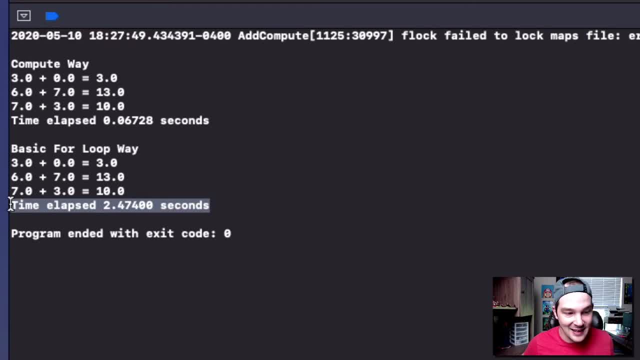 more data to be processed. we're going to get a lot more data to be processed and we're going to get a lot more data to be processed and we're going to get a lot more data to be processed and we're going to get a lot more data to be processed. this number gets a lot bigger. This. 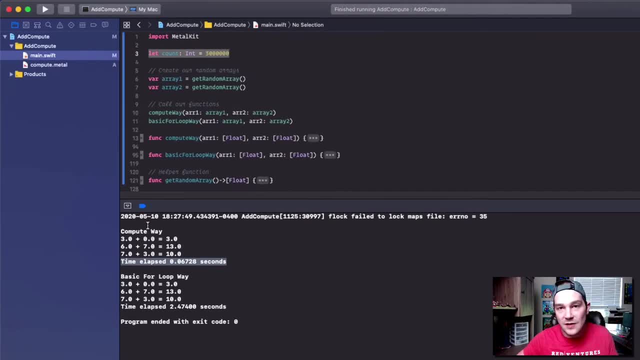 one basically stays the same. So that's where you know we should use a for loop and we should use the GPU. So in this case, I want to show you how to use the GPU. So what I'll do is I will jump. 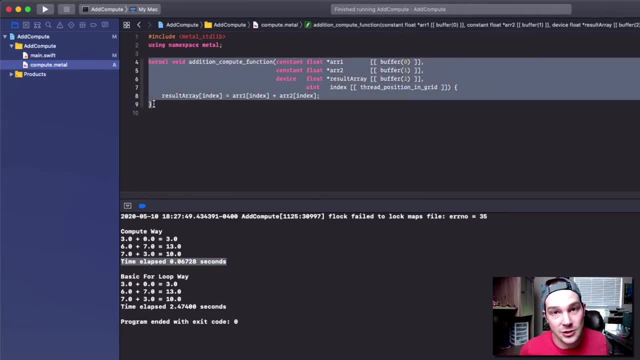 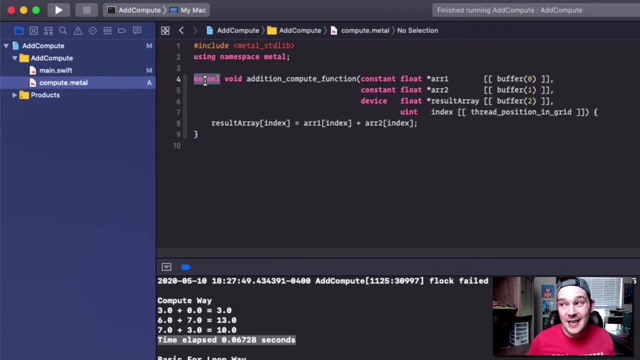 into the computemetal file and we'll talk all about this function. So the first couple of things to note about the function is it says kernel. Kernel means it's a public GPU function that can be accessed and called from the CPU. That's what kernel is, If you've ever done anything with Metal. 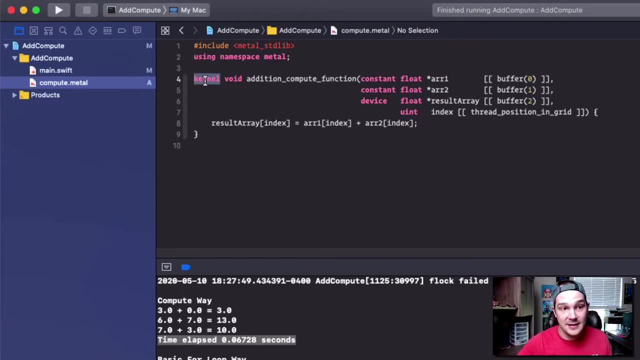 Graphics. if you've ever done anything with Metal Graphics, if you've ever done anything with Metal Graphics, you would know that this might say vertex or fragment. In this case it's kernel. It's just defining what the function is for the CPU to be able to come and access The next thing. 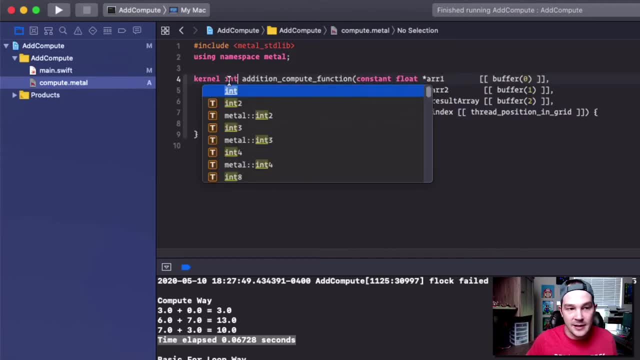 is void. So this you know, you could say int right here because it returns an int. Nope, we don't want that, We want void, because we're not actually going to be returning anything using this kernel function. We're going to be modifying, in this case, this result array and then just the buffer will. 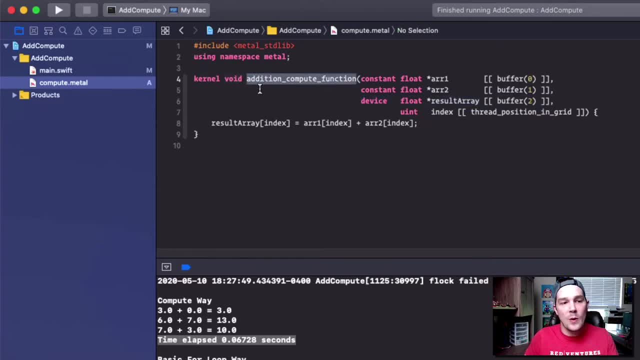 be updated, So we don't actually need to return anything. And then we have this name right here, which is additional, And then we have this name right here, which is additional, And then we have addition compute function. Now this name is really important because over in the mainswift, 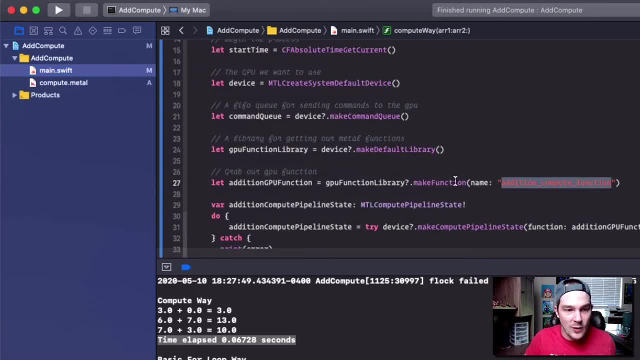 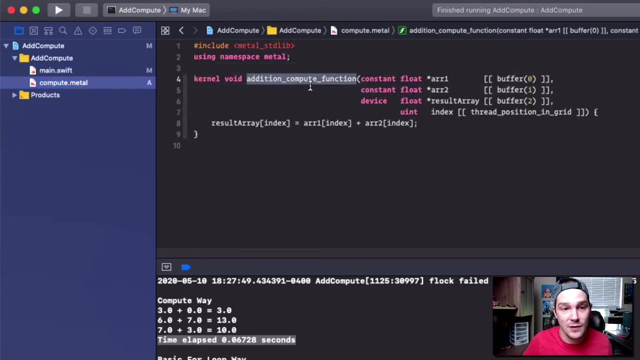 if I were to jump into the compute way really quick, you'll see that we are actually trying. we are actually grabbing this function based on the name of the function, And so that's what this is. This is the addition compute function. The next thing we have inside of this function are: 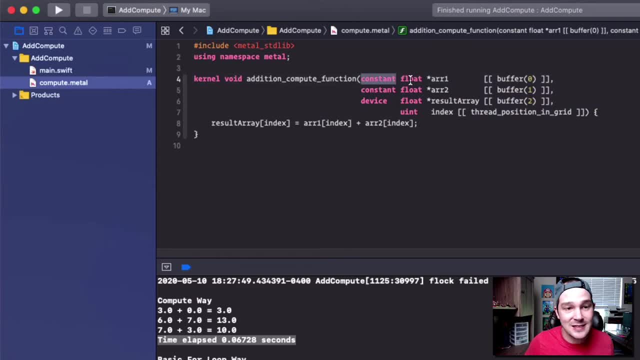 four different parameters, The first parameter being constant float pointer. array one, buffer zero. And then the second one is array two. Now, these are the two arrays that are we are adding together And in order to talk about what this buffer at zero thing means, this gets into how 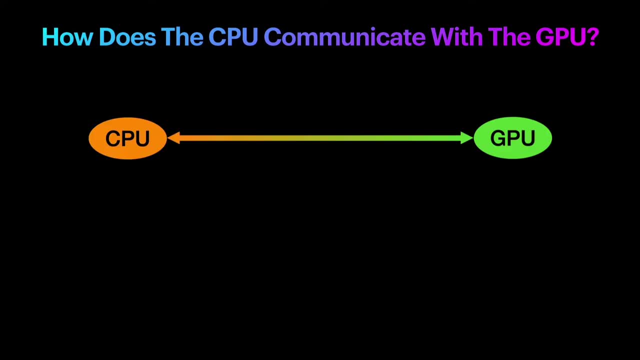 does the CPU communicate with the GPU? Now, you might think that the CPU and the GPU have a direct line of communication. That's not how it works. What you should be thinking is the CPU and the GPU act as separate sources And in between the CPU and the GPU there is this shared CPU GPU. 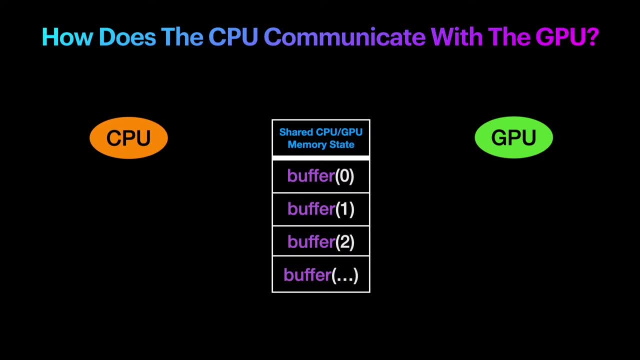 memory state with multiple buffer levels inside of it, So buffer zero, one, two. we've kind of have defined address space And what we do is we basically access that shared memory state from the CPU and the GPU, but they don't actually talk to each other. So the CPU will say: set buffer and 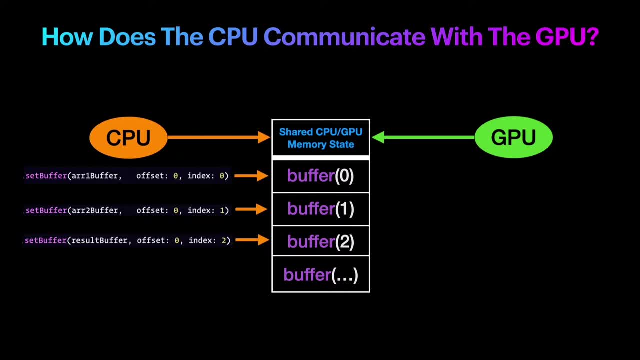 we'll put like array buffer one uh at index zero And it will store that in this shared memory state And then the GPU can then go ahead and read those values by those attributes that we're using in this first function parameter. This is how they communicate. 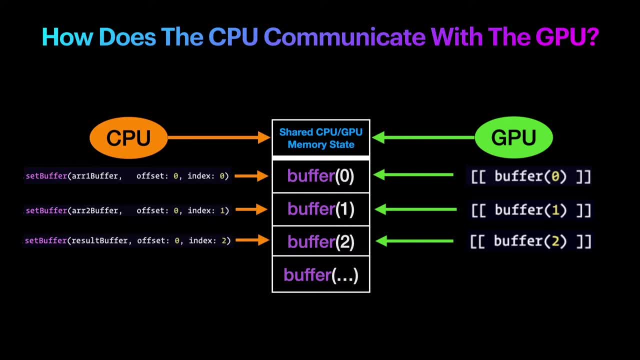 Not just a direct line of communication. This is why metal and open GL, This is why it's stateful, because the CPU and the GPU, they share memory, this memory state. And then when from the CPU we'll say something like I don't know, dispatch threads. And once we dispatch those threads, 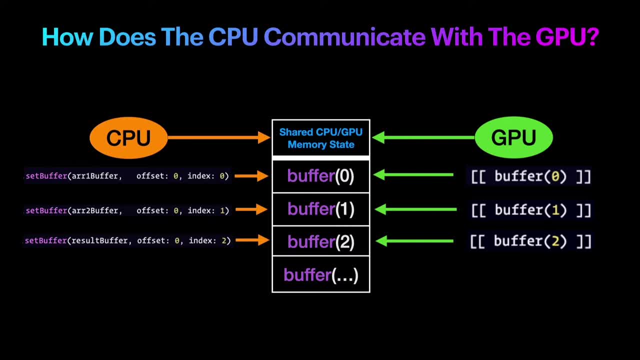 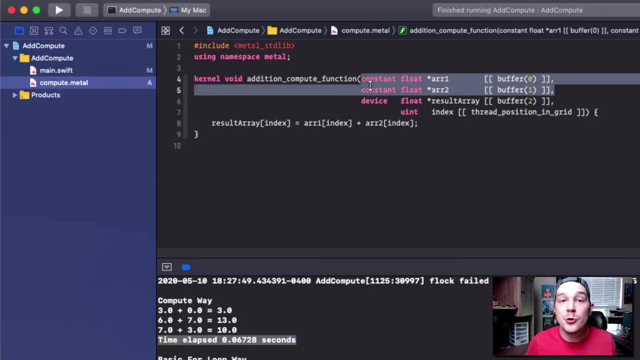 the GPU will then read from this buffer, not you know, Hey, execute the function on the GPU. So that's how the CPU communicates with the GPU and back in the code. Yes, we have the two arrays to add together. Uh, we are using this. 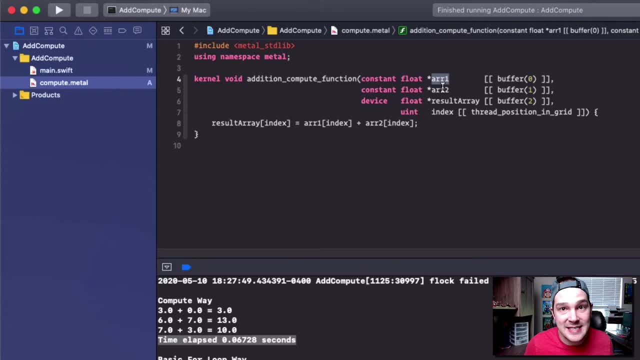 keyword of constant, because we're not actually going to be modifying this data. We're only going to be reading from this value. So we need to make it constant. It's not going to change, However, the result. the race stored at buffer two is going to change. 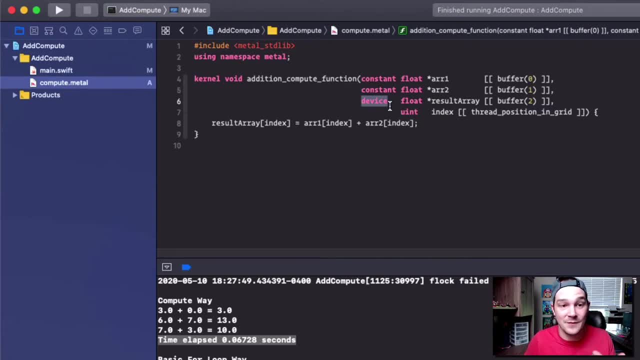 So we're going to use the constant or the keyword of device. So device means that we can write to this buffer and then use it off in the CPU. So that's what this is going to mean. This fourth parameter right here is really cool in that we don't actually need to. 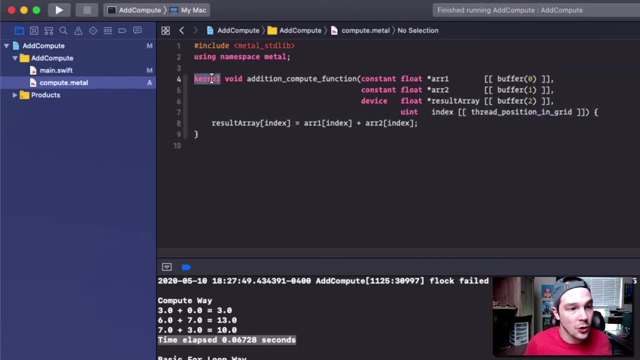 pass in this parameter. This gets tracked per kernel. So when we're using multiple threads, every single thread process it's processes its own kernel function, So the thread itself will pass in this current index. Now I created another keynote presentation to talk all about this function, So check this out. So here is basically the same exact parameter. 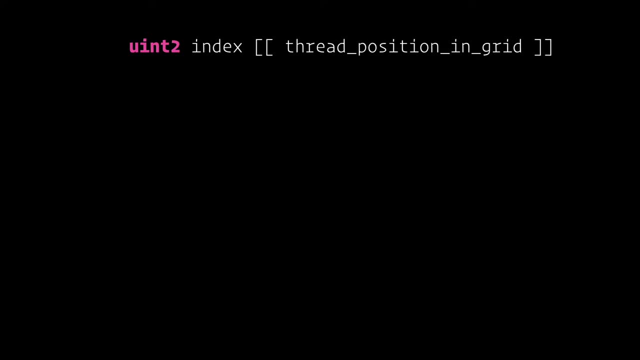 that we were using inside of that function, where we have- you went to index, uh, and then we have this attribute of thread position in grid. Now, the first thing I really want to focus on with this attribute, uh, parameter is grid, So we all know that this, this, this. 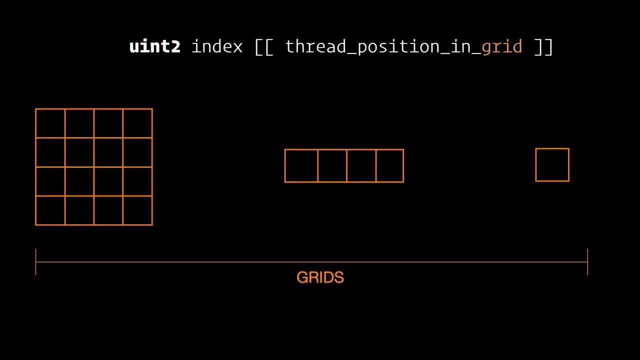 these all equal a grid. These are all grids. Basically, a grid has a width and a height. In this case, it's a four by four: four width, four height. We have a four width and a one height here And we have a one by one. These are all grids. When it comes to a grid, we know that. 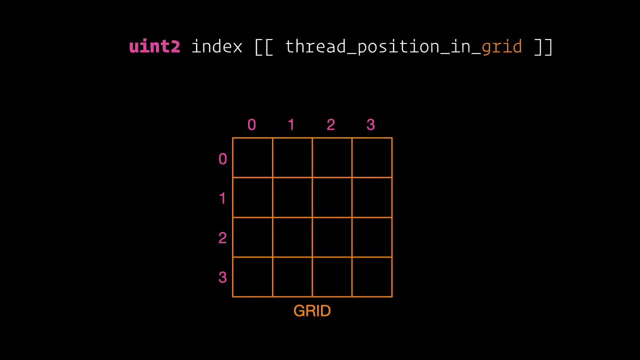 this grid will have index positions, Okay, And inside of these index positions we have threads. So basically, each one of these teas represents our operation. In our case, we're adding two arrays together, So we have a plus B. what values are we adding together currently? 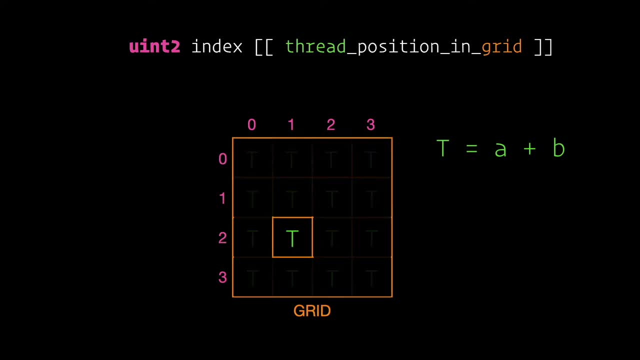 in that thread. So say, we were to focus on this little box right here. Well, now we have the thread position in grid, which is a Uint2.. So we could say that this actual index is one two, because it's at width of one and height of two. So this index literally represents the location. 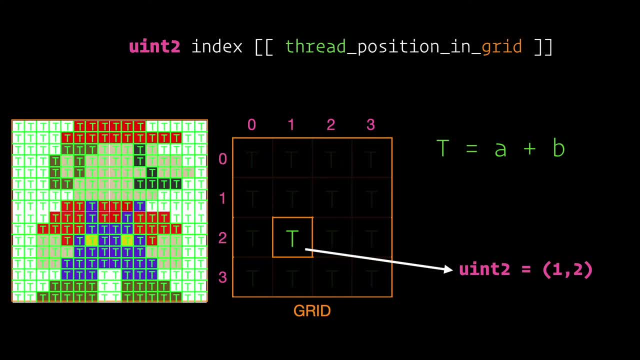 of the current thread we are processing. Now this is really good if we are processing something like an image, where an image, every single pixel, represents one thread and we're doing an operation on that pixel. Basically, we can access whatever pixel we currently want based on this thread position. 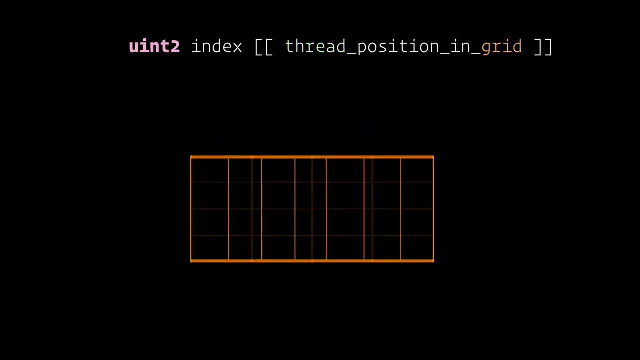 However, we are not working with images. We are working with a simple one dimensional array of numbers, And each one of these operations is A plus B. This array at index plus array at index is basically one individual thread. In this case, we have a seven by one grid, which means we don't 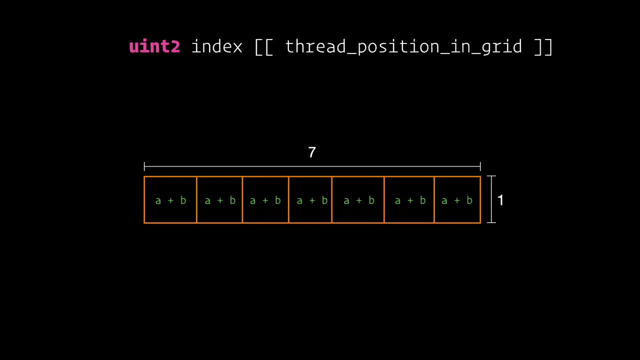 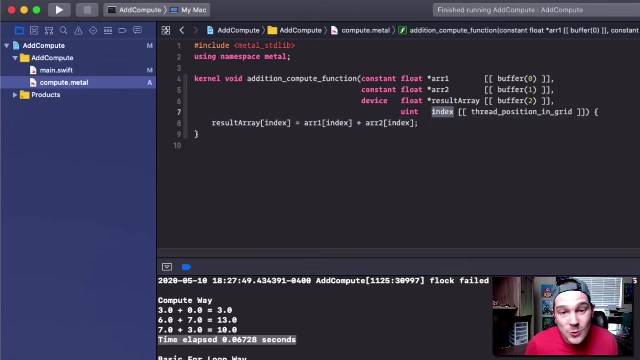 need a Uint2 because it has a height of one. Really, all we really need is a Uint. We don't need that extra height parameter. So when we're calling Uint index thread positioning grid, we're basically just accessing that current index And now back in the code we can use this index. 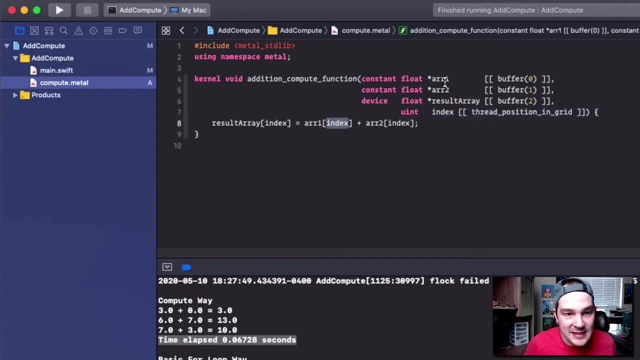 at that current thread to then access each one of these arrays. So, as you can see, the only code that exists inside of this function is to store at result array, at this current index, the value of array one at the current index plus array two at the current index. 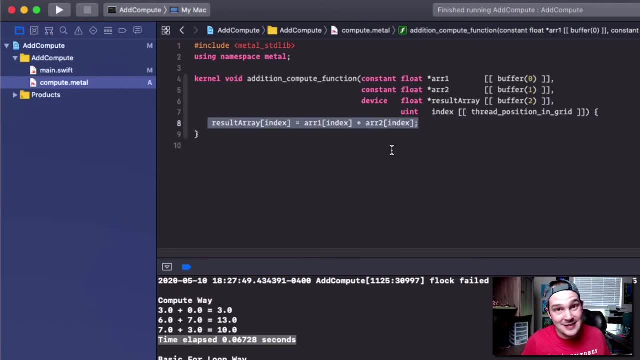 And since this all happens on multiple threads and each thread tracks itself, we don't actually need a for loop here. This is our for loop. We are automatically having a for loop without having a for loop, So that's pretty cool. Now that the GPU functions all talked about. 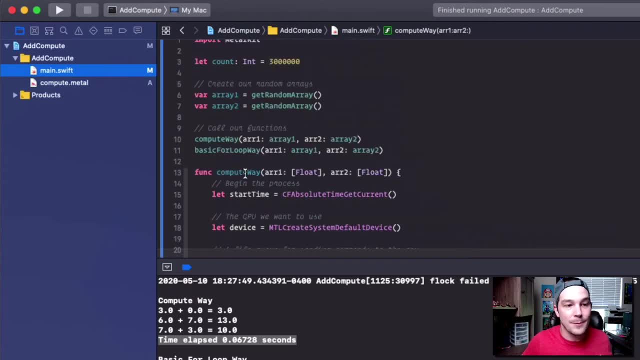 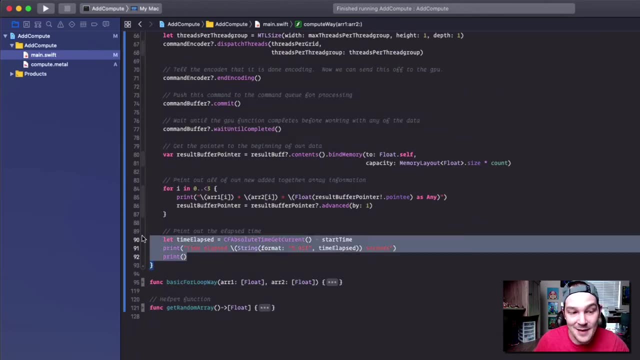 we can go back to the Swift file and talk about all of this compute wave function. So the compute wave function starts off by basically getting that exact same start time And at the very end down track the time elapsed. So that's kind of what happens. We want to benchmark to compare. 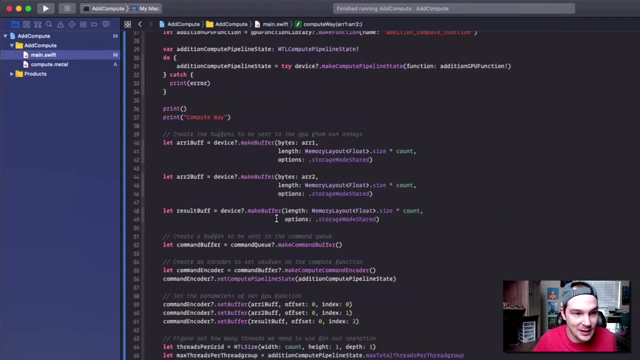 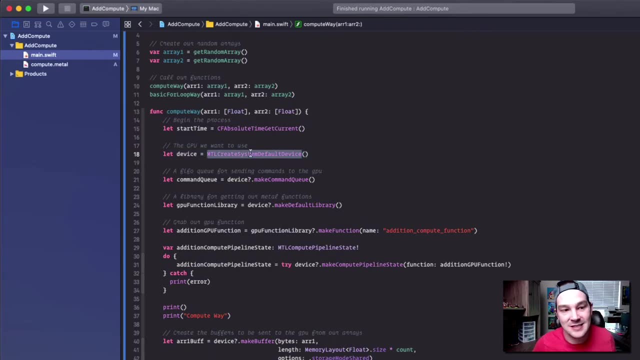 as you can see down here with these printed out statements, that's just the time elapsed, And then we go on to actually using the GPU. Now the first thing we call is: let device equal MTL, create system default device, Basically, if your computer has multiple GPUs on it. 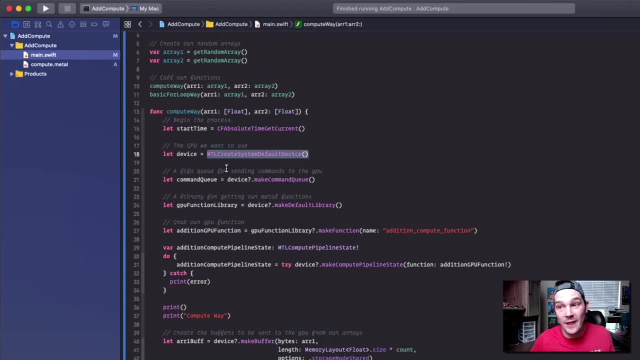 we can actually select which GPU we want to use for that current operation. In this case, my computer only has one GPU, one dedicated GPU, And so using this function is sufficient. Underneath that we have this command queue. We can't just call GPU functions Like I. 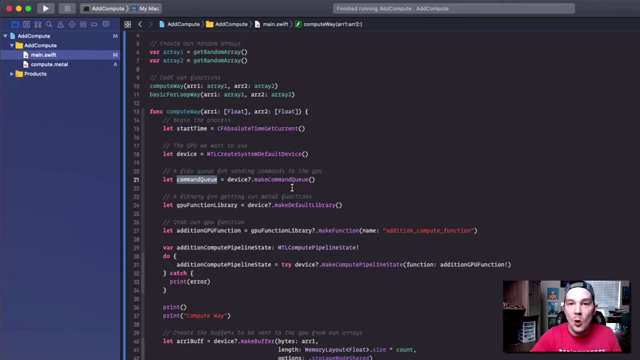 said before, there's no direct line of communications. but what we can do is we can set up a command queue that we can send commands to and it will process it first in, first out. Then the next thing we do is we grab, we use this, make default library from the device. 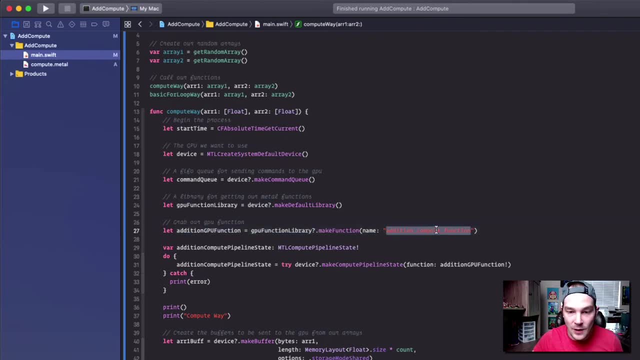 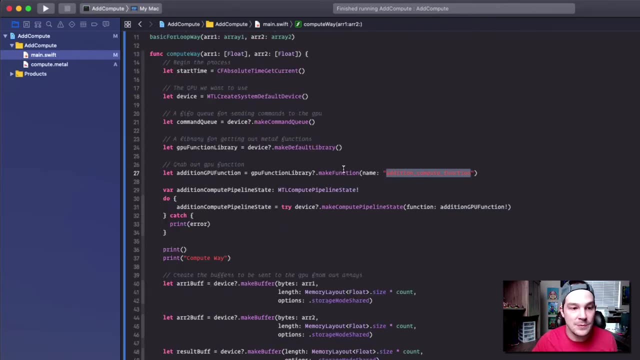 and we use that library to find our metal function that we created already. So this right here represents our exact function that we wrote on the GPU. Now we can't just have a function- Oh, that'd be way too easy. What we actually need is we need some sort of a compute. 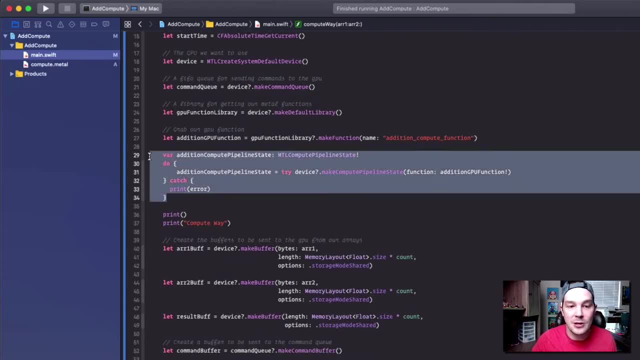 pipeline state. So the next thing I've done is I've created this compute pipeline state, And the reasoning behind this is because, like I said, the data is stateful, And so this pipeline needs to be a stateful pipeline, not just a function that we can call over and over again. 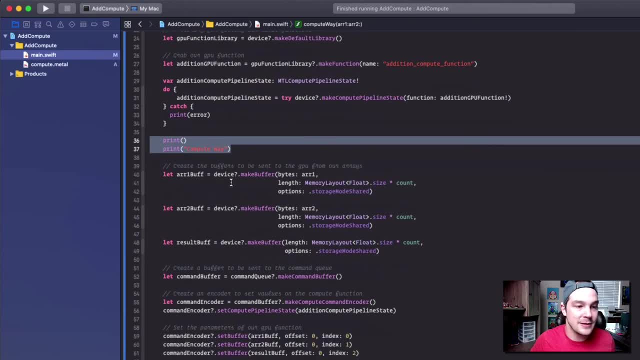 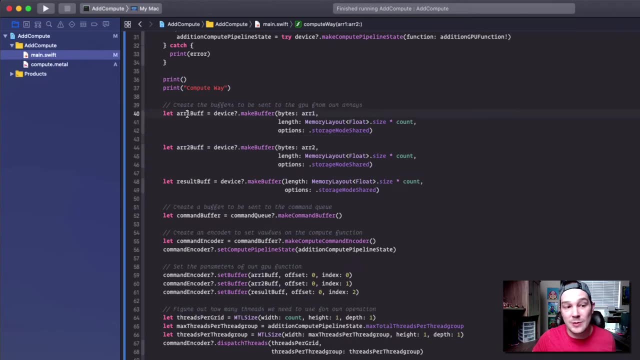 So that's why there's a pipeline state Going down to the next step. we're going to go ahead and do a little printing to make it look a little clean, And then we create these buffers that we pass in as parameters. Now, the first one is going to be array one buffer based on array one that we 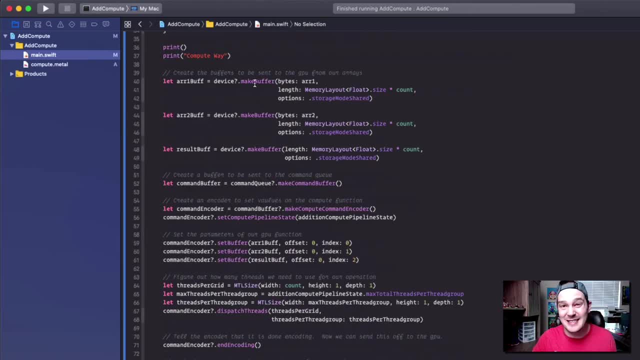 created up here at the top. So we're just going to generate what's known as an MTL buffer from that array And then we're going to create another array buffer, So this will be array two buffer, based on the second array. So basically, what we're doing is we're just allocating this MTL. 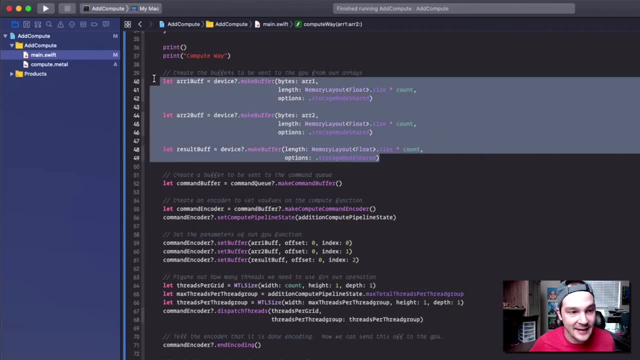 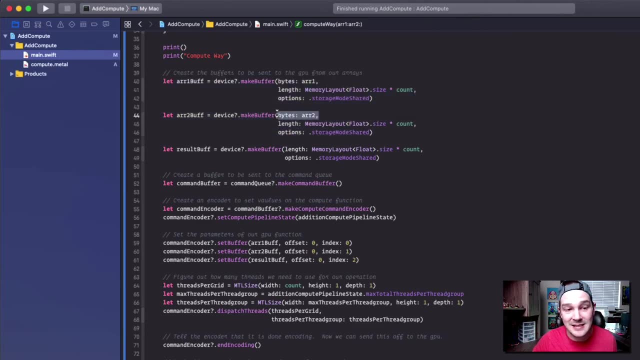 buffer memory to be able to be passed to the GPU, And we do that with these three functions. Now, this third one is a little bit different than the first two, and that's because we're not actually using bytes to generate this result buffer array. 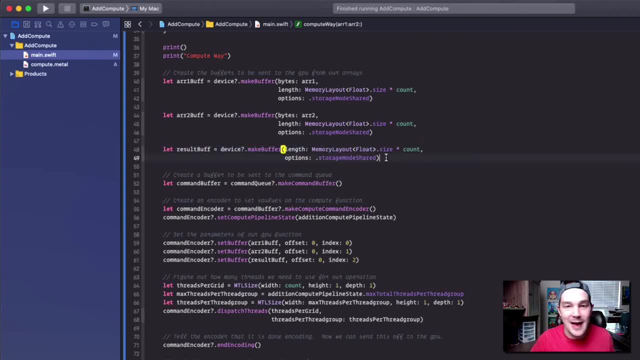 Since we're going to be only writing to this array, this can just be allocated space. It doesn't actually need to be any numbers, any zeros, pre-allocated. All it needs to do is just be an open memory slot, open buffer to be able to write values to from the GPU Going down. 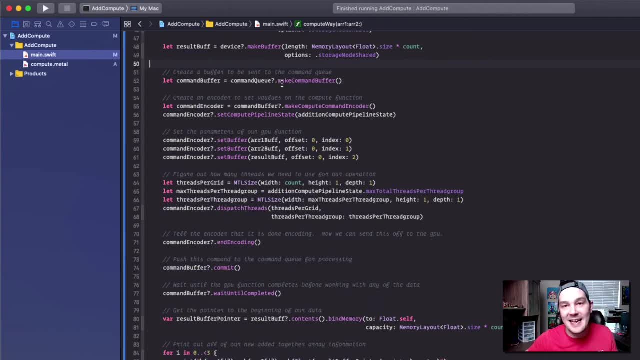 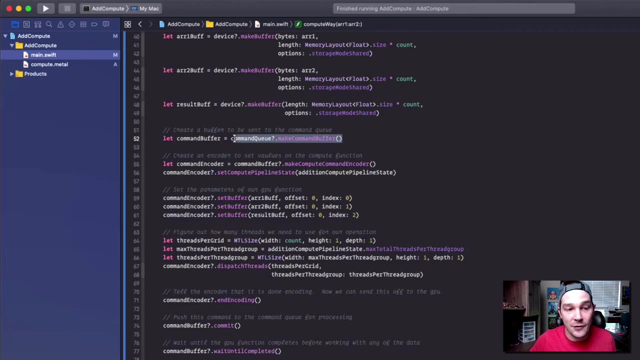 we are actually going to start by. we're going to start sending our function to the GPU, and we do that by creating a command buffer, And we do so with that command queue that we created above. Basically, we use this command queue to say: Hey, I need a command buffer to be. 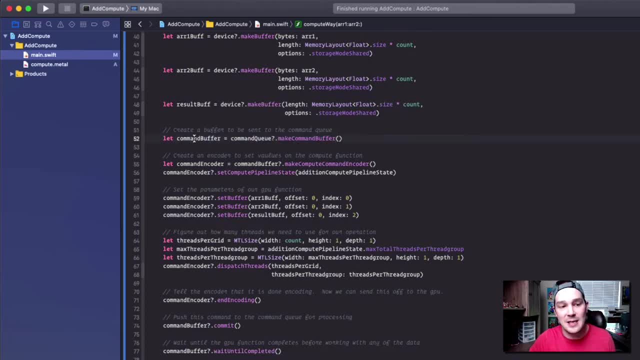 able to send to you. It's allocating room for this buffer. So we're going to create this command buffer. Now, in order to encode the command buffer, we need to create a command encoder, And that's simply by calling command buffer dot. make compute command encoder The command. 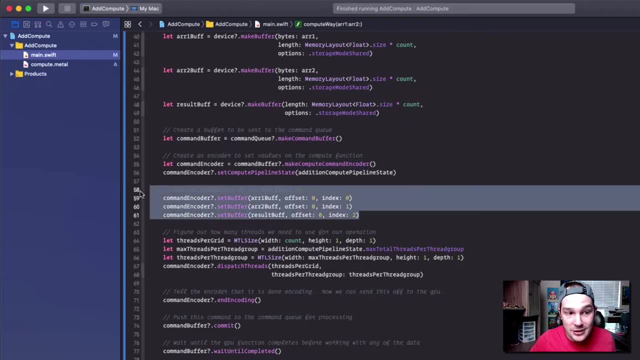 encoder's job is to basically set these parameters, And then we're going to create a command buffer. Um, I'll get to that in just a second. Before we do that, though, we say command encoder dot. set compute pipeline state to the addition compute pipeline state that we've created with that. 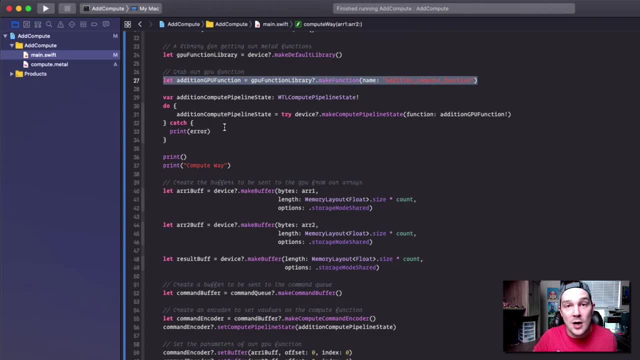 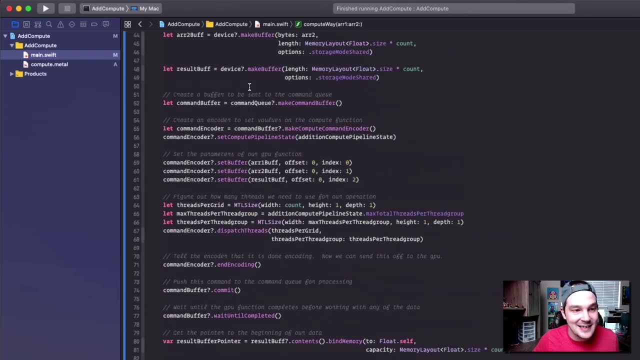 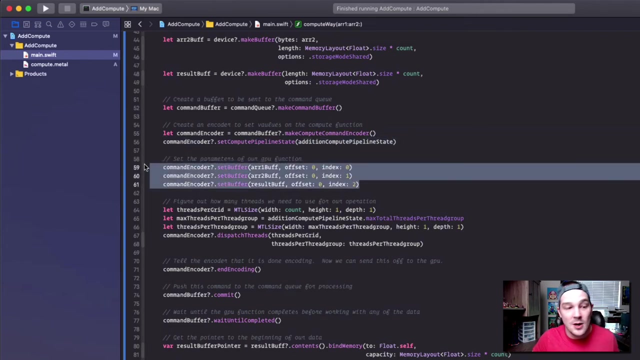 addition GPU function. So now it knows this is the function we're going to be using during all of this stateful processes. So we said: command encoder, dot set- wait, where'd I go? dot set compute pipeline state to that addition compute pipeline state. The next thing I do, like I said, is we add: 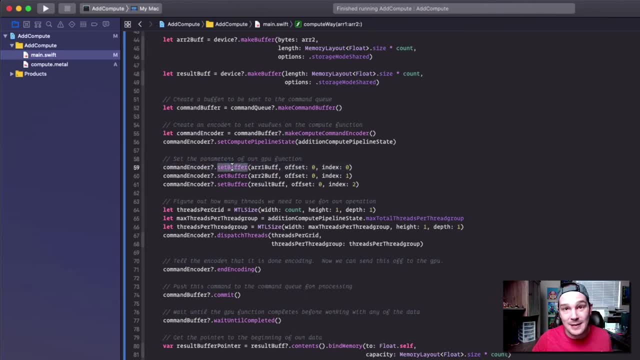 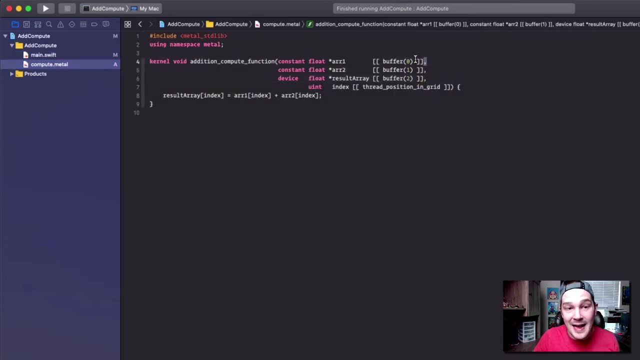 these as parameters. Now we say command encoder, dot, set buffer. Just like I said before. we say set buffer, the first buffer offset zero at index zero. So if I go to the compute dot metal, I am setting this parameter right there with this function. I'm doing the same thing with that. 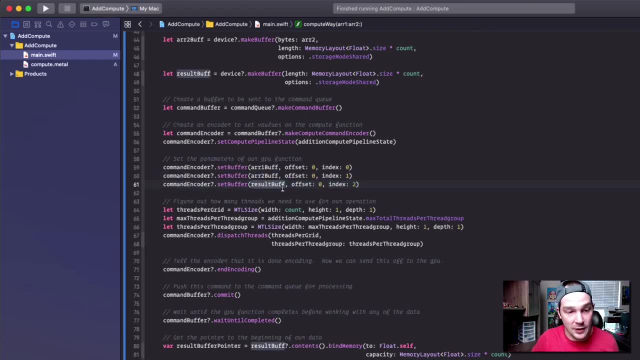 second buffer and the third thing with that result buffer, And I'm setting those all with the relational uh index right here: zero one two, zero one two. So that's where I'm encoding those parameters. The next thing I'm going to do 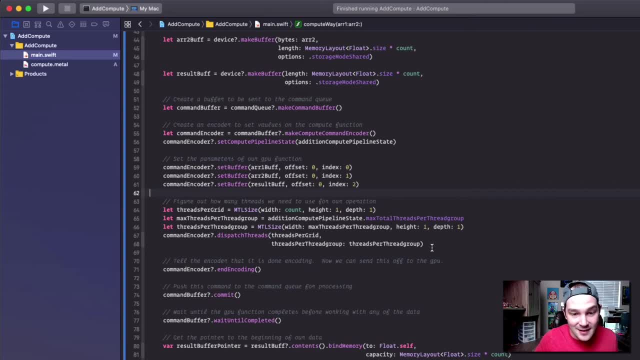 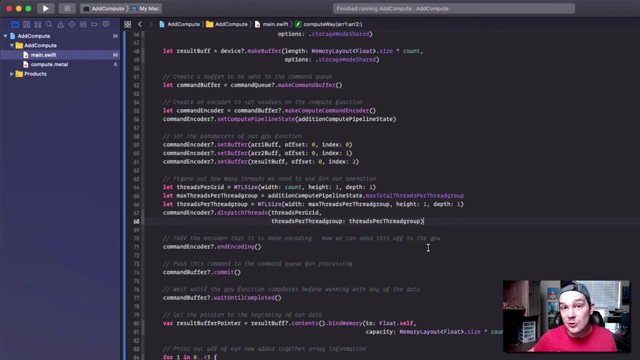 Actually going to want to dispatch all of the threads that we need. Okay, So that's what we're doing. Uh, based on our array, our computer has no idea how many threads we're going to need for this operation, So we need to tell it: this is how many threads we're going to need. This is how many. 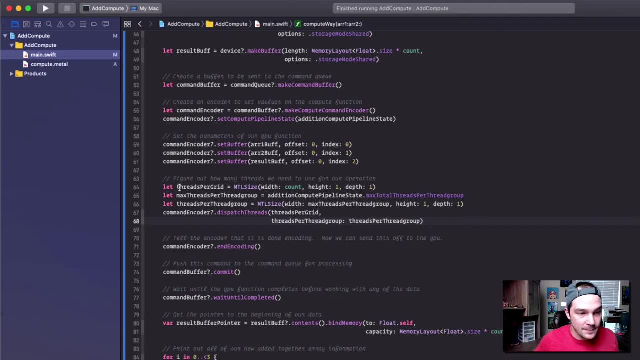 of those indices we're going to need to populate, And so what I've done here is the first thing to kind of note is this final function. So these are just variables building up to this final function. command, encoder, dot, dispatch threads. The first thing we need to tell it is the threads. 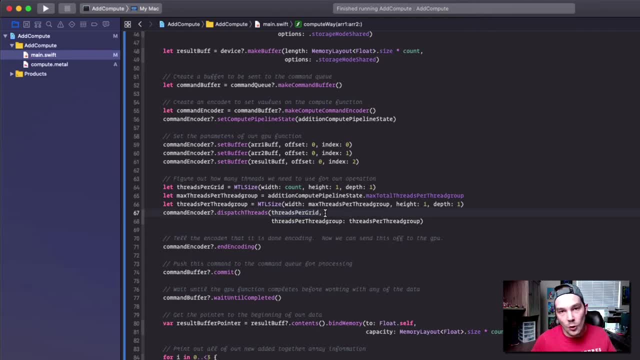 per grid. So when we talked about the grid, we talked about four by four. that would be about 16 threads, right, Because four times four is 16.. That's the area, So we would need 16 threads per grid. Now, something to note, though, is it is of MTL size, which has width, height and depth. 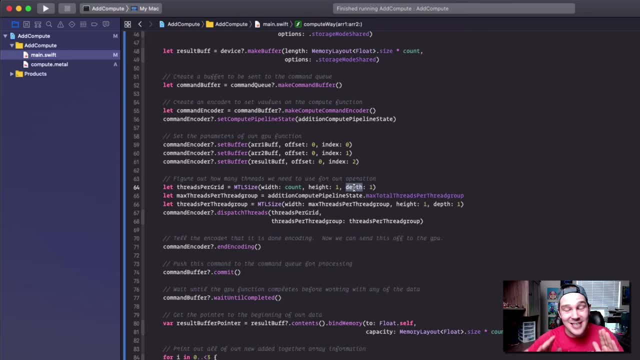 which means that our threads can be not one dimension, not two dimension. We can have three dimensional threads, which is amazing. Please implement something with three dimensional threads, something like an octree. Just go off and do it please, Cause I want to. 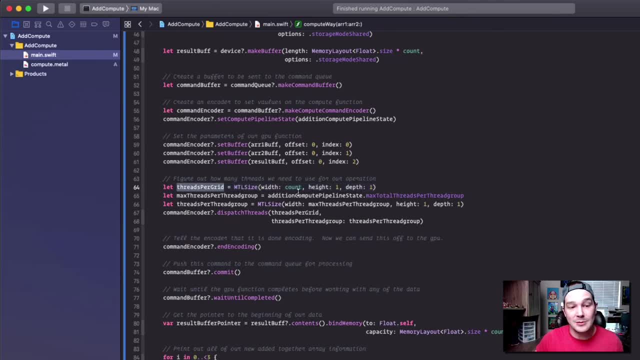 see it, Um, and I think that's super cool. So basically, what I'm just saying is this: threads per grid. since we don't have a height, we are working with a count by one. So, like width, width by height, count by one one height, uh, we only need to operate on the width. 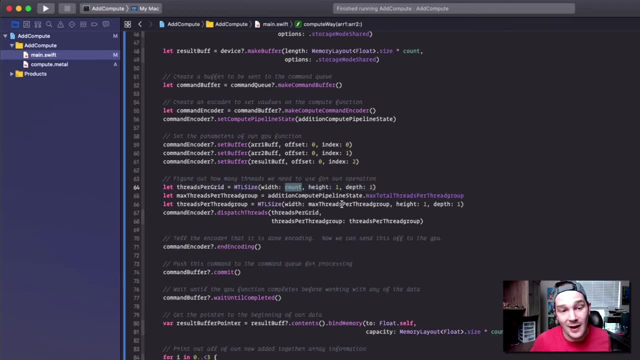 So we need to set threads per grid equal to a width of the count of our array, And then this max threads per thread group. this one's a little bit more complicated, So your computer cannot process Okay. Okay, So you can only process infinite numbers of threads at one time. It can only operate on a certain. 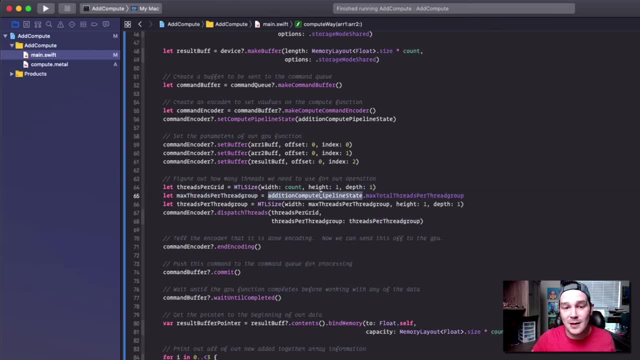 number When you call this function. basically I'm using that compute pipeline state to get the max total threads per thread group. This value will return how many threads you can store in one thread group, And a thread group is basically all of these threads will execute, Then the next group. 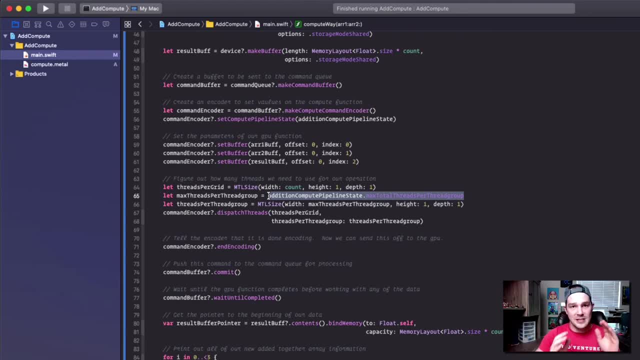 will go, then the next group will, then the next group. If your thread group is a two by two, it's only going to process four at a time, because that's two times two, So four, uh, three threads will go. four threads will go. four threads will go. four threads will go When I call this. 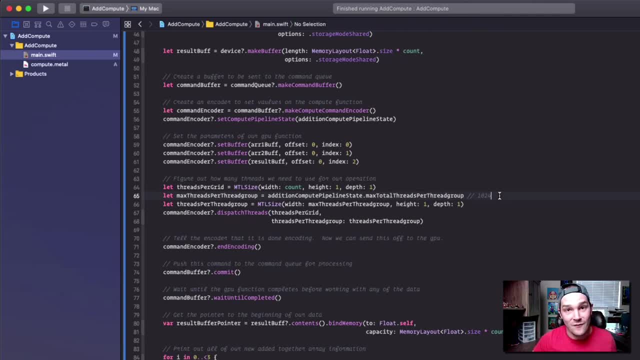 function. this for my computer returns 1,024, which, if we had like a texture, uh, we can have a width of 32 and a height of 32, because that equals 1,024.. In my case, with this, max threads per thread. 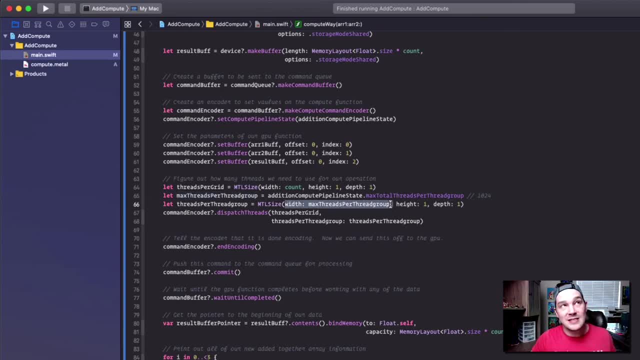 group. I'm just passing that in as the width. So in every single thread group we can have 1,024 threads in that thread group. I hope that made sense. If this doesn't make any sense, I have a discord channel. I have a. 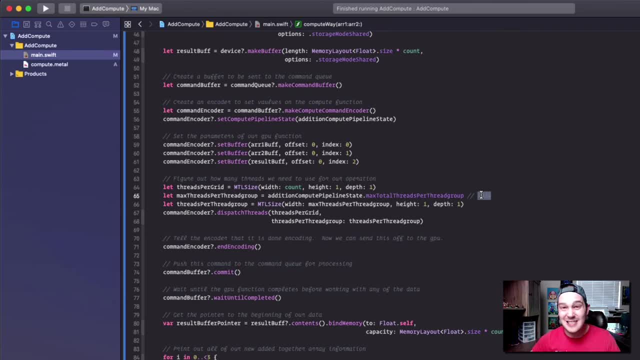 comment section, just comment. I will answer that question. This is some tricky stuff And I want you to understand it because it's really cool. But basically now we have this threads per thread group, all the threads that we can store per thread group, And we store that here. 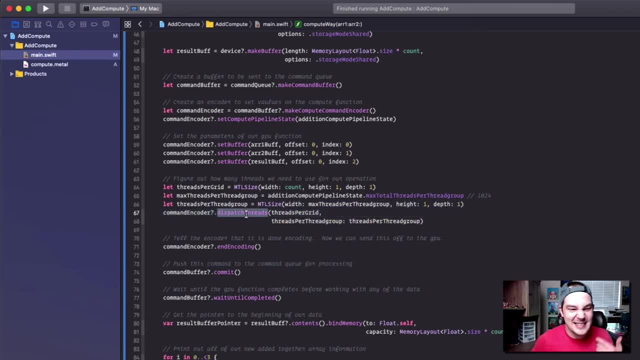 Now this dispatch thread- in my mind it used to be- this is the function call. This is not the function call. This is just saying, like when we dispatch the threads, this is how many we need. The thing that calls the function is something down here. So we need to tell the command and 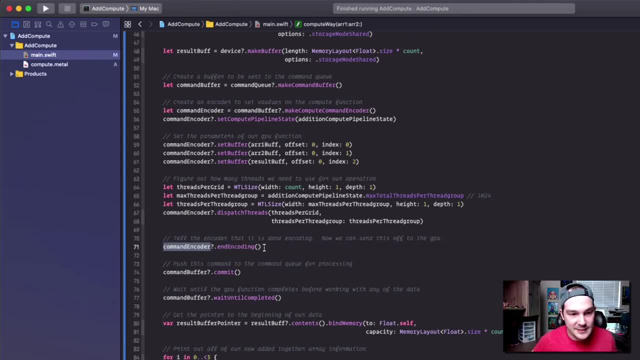 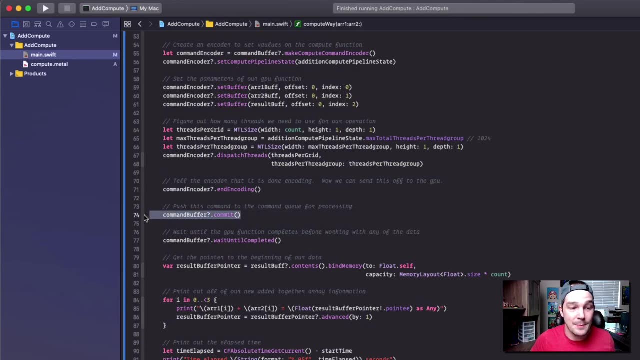 encoder to stop encoding. We are done encoding. After this point we cannot add any more things to this compute encoder or to this command encoder. And then we call this command buffercommit. Now this function right here is what sends it to that command queue. Now that command queue will process. 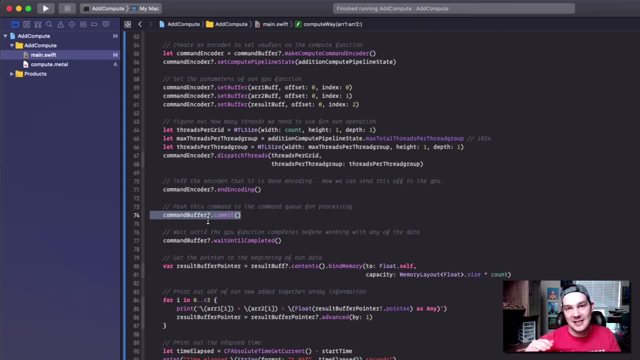 the second. it gets the newest command buffer. it will process it And we can build up a backlog of all sorts of command buffers. But in this case we're just going to say command buffercommit. It's going to submit this one command buffer. There's not any other command buffers to be. 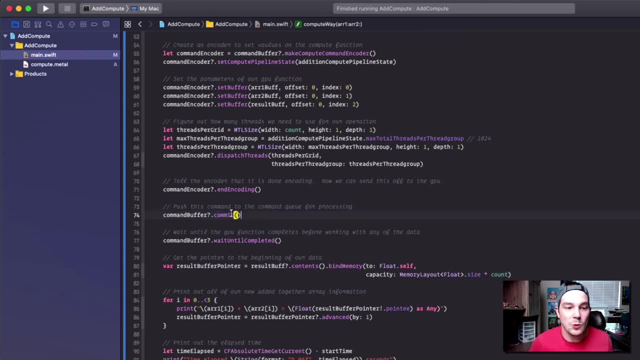 added. We could do some after this, but it doesn't matter. This will basically execute that function as soon as it gets to the command queue Underneath that we call wait until complete- completed, because now we want to kind of print out all the resulting numbers that have been added together from those. 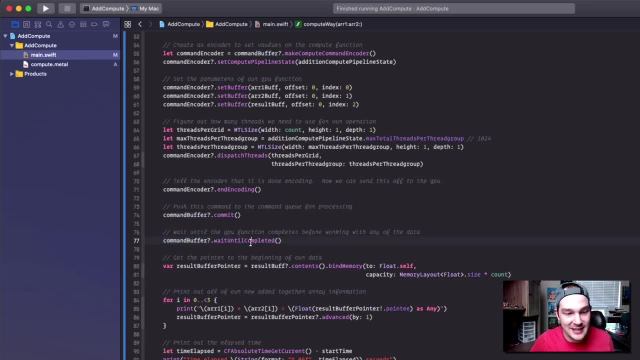 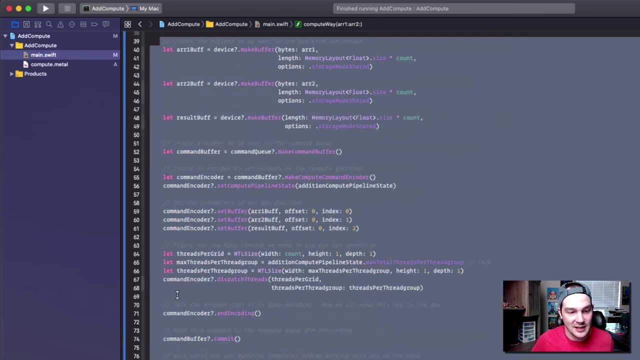 two buffers, And so we need to wait until this command buffer completes, or it's going to get to these lines and that command buffer is going to be empty, So it needs to wait till it's done processing, because this is somewhat of a background process. Actually, it is a background process. 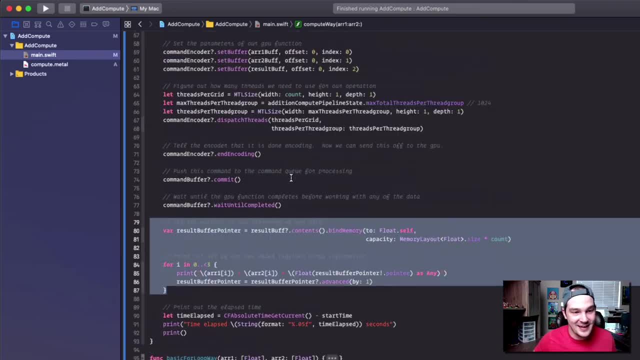 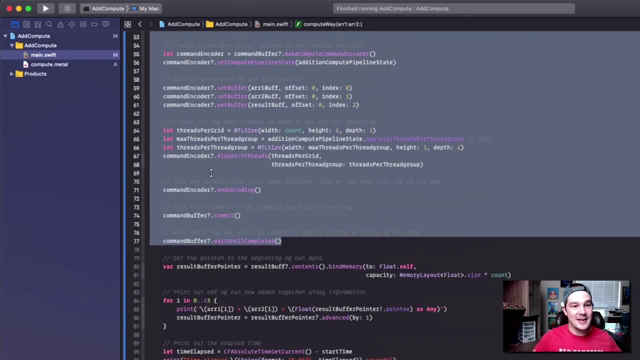 Uh, and then finally, uh, after, so, we, so, so we've done it. Uh, we send, using these lines right here, I guess let's go up to the top using all these lines right here. It's a little bit more. 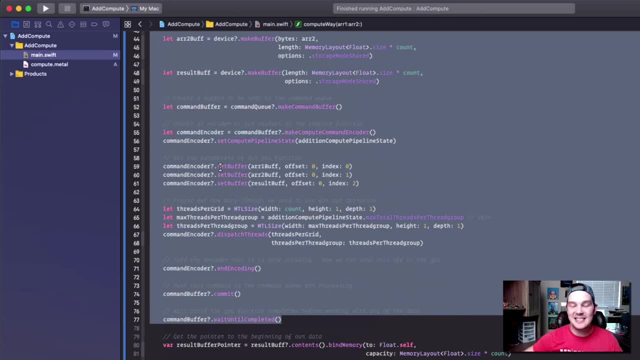 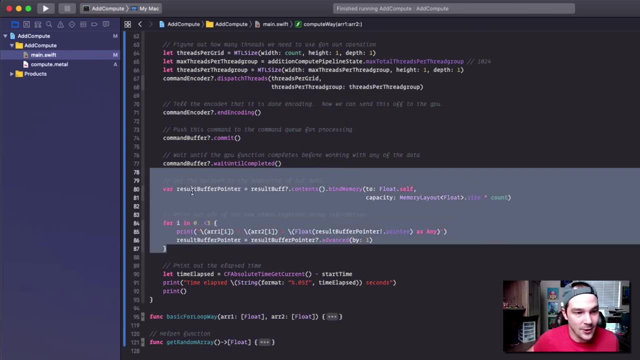 complicated than that for loop, but we have successfully sent off to the GPU to do some processing Uh, and underneath here is just basically printing out those results. So what we do is we get this result, buffer pointer, and this function right here will basically use that result. 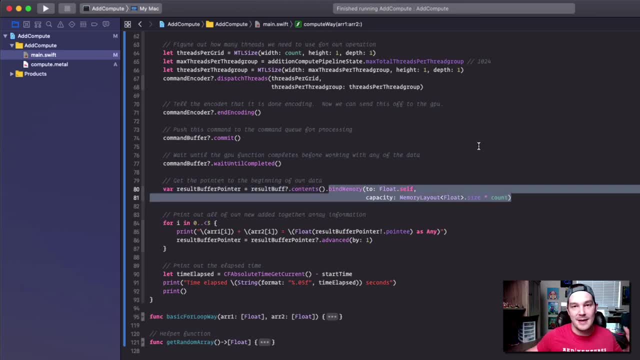 buffer pointer. It will grab the contents and bind the memory to this basically big allocated memory on your CPU And it will point to the very first value, And it's actually a pointer to that very first value, So it's like the first memory location of that, Anyway. uh, this is basically. 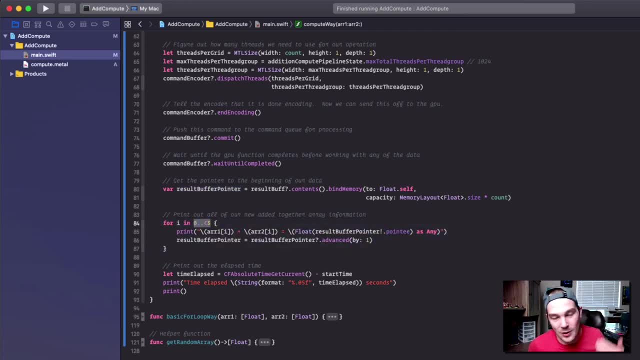 the first value And then underneath we're iterating through only three values, Cause I only want to print out three. I don't want to print out 3 million. Uh, and I'm printing out. array at I plus a Ray two at I equals. 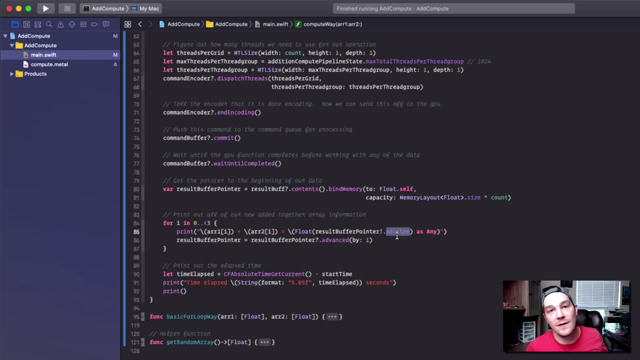 buffer pointer dot pointee. this pointee returns the float value that is at that current location. or if it's not a float array, it could be whatever you want, but in our case it's a float, and yes, then i use this little function to increment that result. buffer pointer to the next value, and yeah. 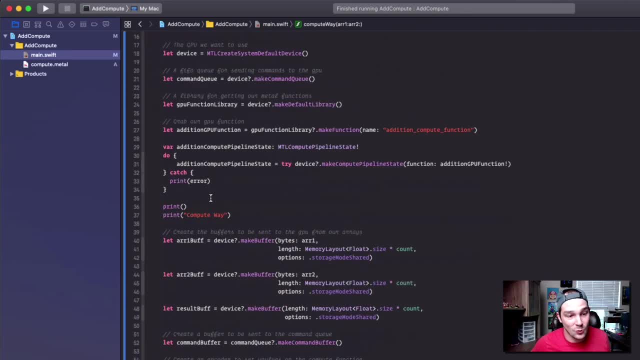 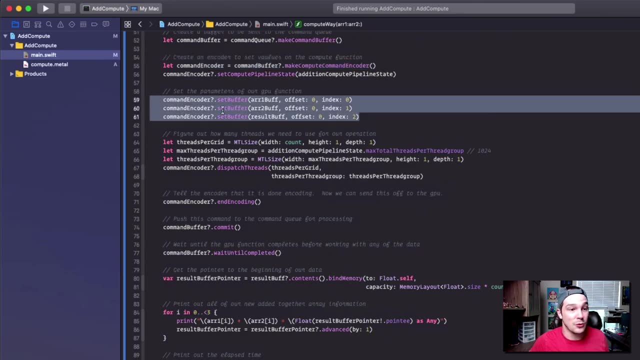 that that's it. that's how this compute wave function works. it basically creates buffers. it creates this command buffer and a compute uh command encoder. it encodes all those parameters. it then says: this is how many threads that i need to use, and then it pushes it off, and then it uses.